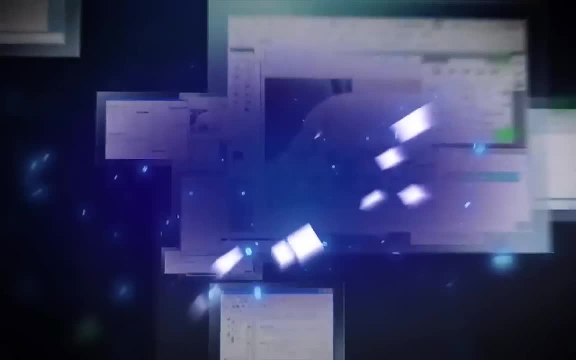 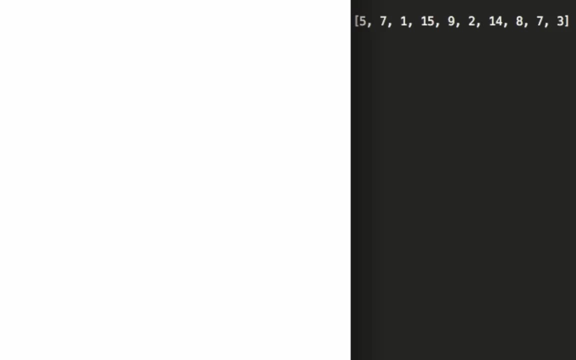 In some past videos, I've talked about binary search trees and how to put them together. However, I took a data set that was very well structured and so the tree was nice and balanced, and then in some of our other videos, we went over red black trees and how to balance a tree that wasn't really structured the way. 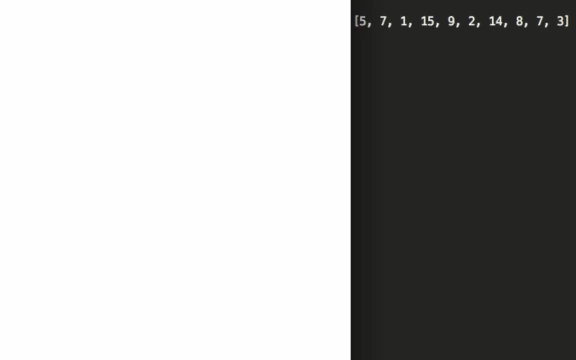 you'd want a red black tree to be structured. In this video I'm going to show you how you can take an array and how you create or construct a binary search tree based on the elements of that array in their original order. So you can see, on the right hand side here we have an array with elements 5,, 7,, 1,, 15,. 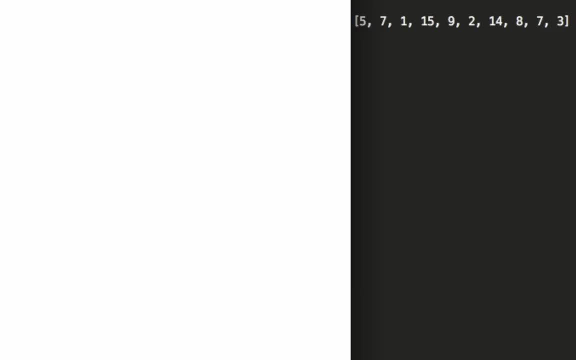 9,, 2,, 14,, 8,, 7, and 3, and so if we're going to create a binary search tree with this array, they have to actually go in order, and so I'm going to show you how that works. So the first element in our array is gonna be 5, and so it's a nice. 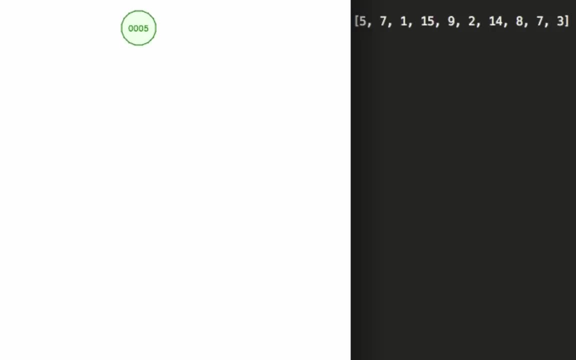 easy. we create 5 and put it inside of the at the root node. The next one we're going to use is going to be 7, and because 7 is greater than 5, it'll do that comparison and then it will put 7 on the right hand side, right. 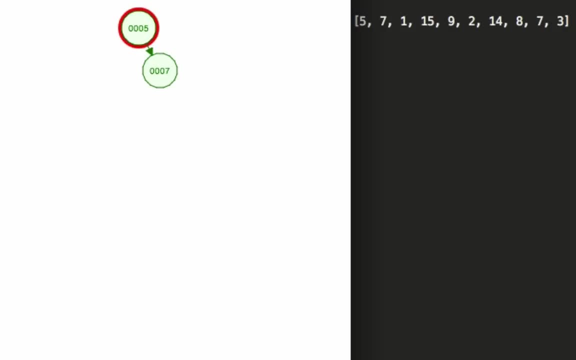 next to 5.. After that we have a 1.. 1 is less than 5, so it goes to the left and right. here we have a very nice basic tree structure. We have our root node, we have 1 being the item or the node to the left, 7 to the right. So far, everything is. 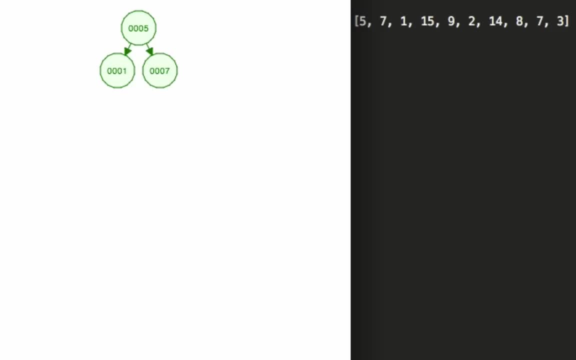 normal. Now we're going to add 15.. 15 is greater than 5.. It's greater than 7, so it needs to go all the way to the right. Now I'm just gonna start adding some more, in order in the array. So we go: 5, 7, 15.. 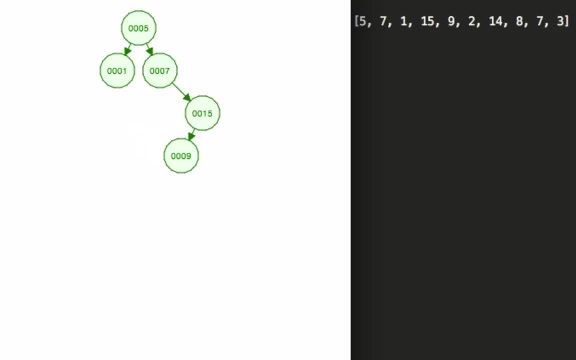 Now 9 is less than 15, and so we put it there on the left. Now, if you are familiar with red black trees or some of these more self-balancing trees, you would know that this is not the way this would have been constructed. It would. 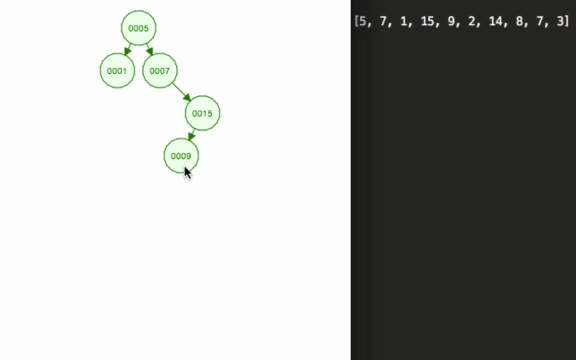 have rebalanced itself and would have swapped out the 9 right here, so the 9 would be connected to the 5.. The 7 would be on the left hand side, 15 on the right hand side. However, this is just a regular binary search tree, so we have to treat. 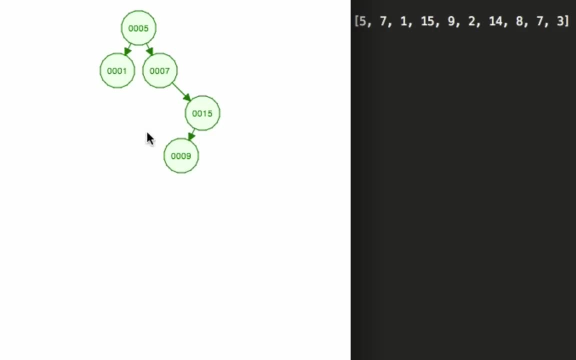 it as such and we have to add the elements in order. And this is a reason why people created things like red black trees was because, as you'll see here in a minute, this tree is gonna look pretty odd in a while, maybe not. We'll make it look a little bit more odd in a matter of 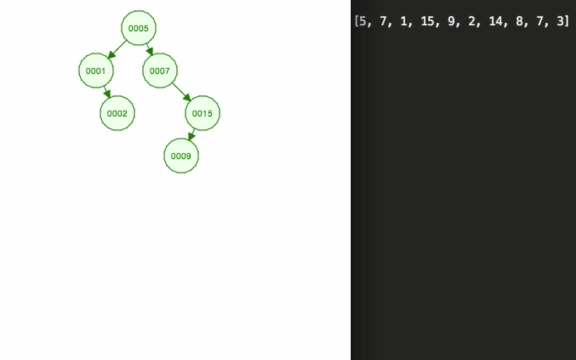 time. So next element is 2.. 2 is less than 5, so we know it goes to the left. It's greater than 1, so we'll get pulled over into the right. Then we're gonna add 14.. It's greater than 5,, greater than 7, but less than 15, so it's gonna move to the 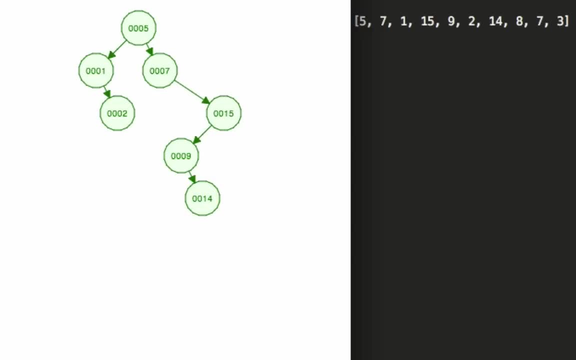 left and it's greater than 9, so you'll see that moves all the way to the bottom of our binary search tree 8.. It's going to traverse the tree. We see that it's greater than 7, but less than 15 and less. 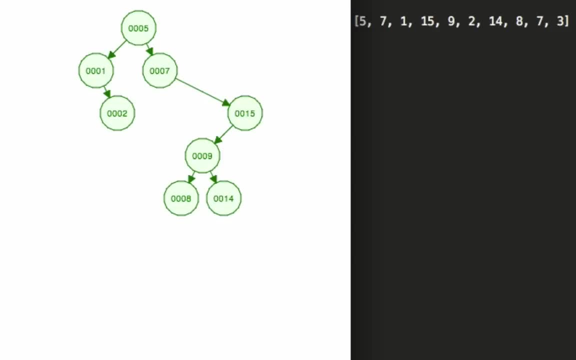 than 9.. And our last, or second to last one is 7.. Now that 7 is an interesting one because you can see that it is greater than 5. It's actually equal than 7, but because it's equal to 7, it's not less. 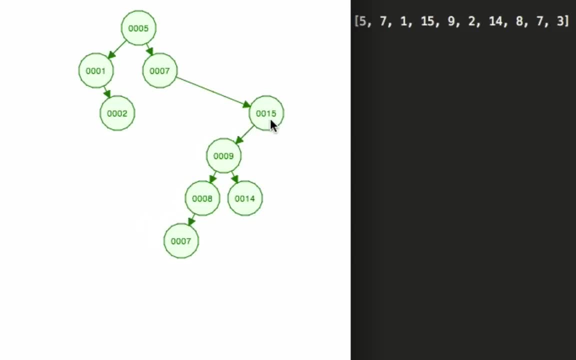 than 7.. It gets moved, It goes to the right, It's less than 15,, less than 9,, less than 8, and it goes right here. So, even though these two nodes are actually the same value, one is directly descendant. 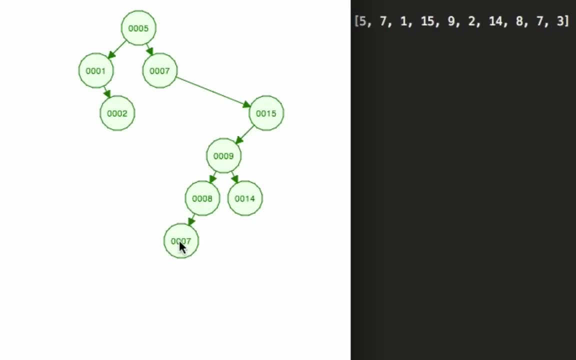 of the root node and the other one is all the way here. Now it is the closest node to this 7 because they are equal, and so it's neat To see the way that that automatically happens. but it's still pretty important to see that you. 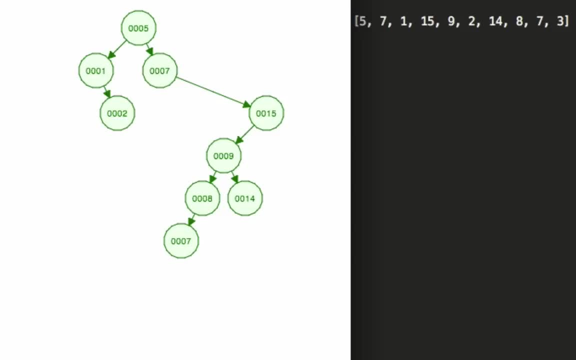 can have a tree that is structured like this, if you take everything in order, And the last one we're going to do is a 3, and that's greater than 1,, greater than 2, so it gets pulled here, And so, given this data structure here on the right hand side, this is what a visual representation of the